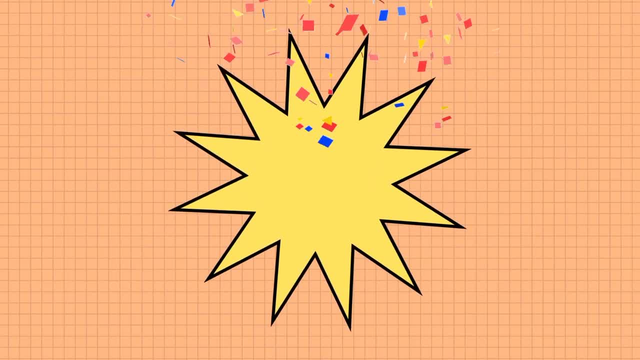 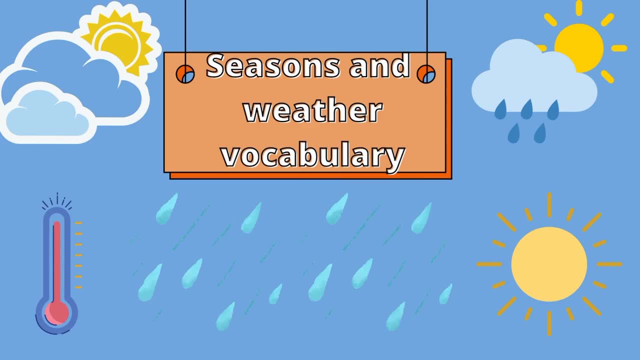 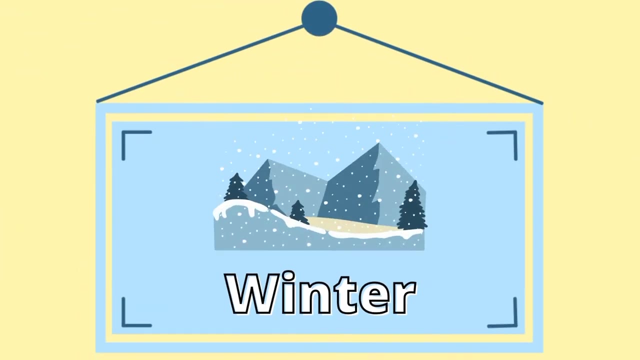 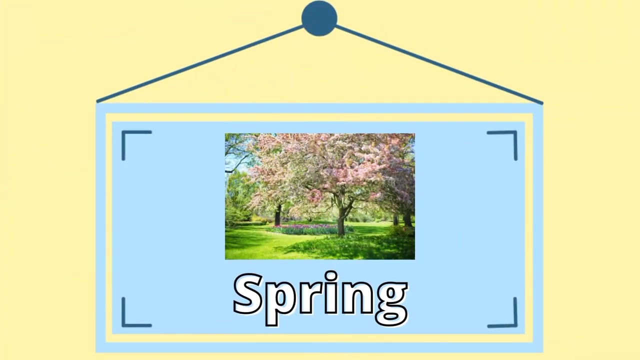 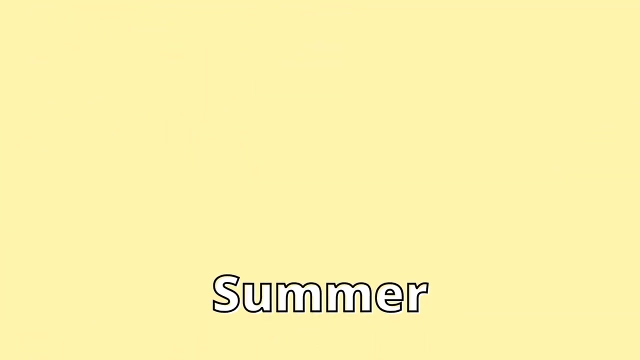 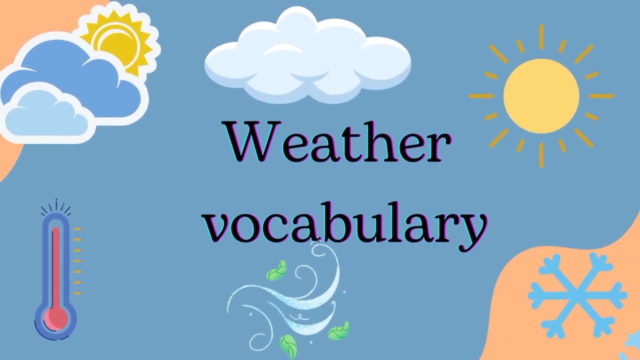 English club. Welcome back to online English club. Let's learn about seasons and weather. There are four seasons in a year: winter- It is winter. spring- It is spring. summer, summer- It is summer. autumn: autumn- It is autumn. Let's learn about the weather. 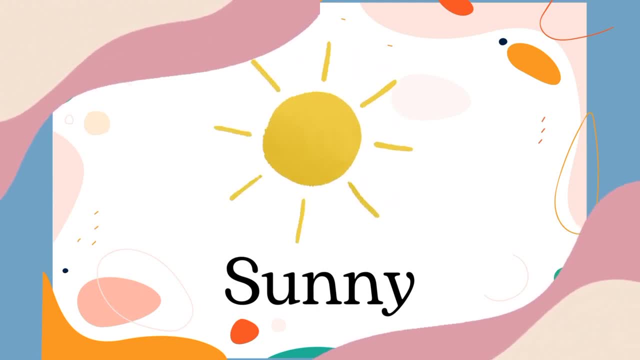 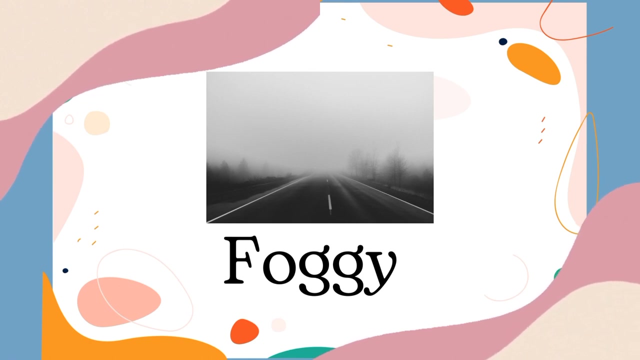 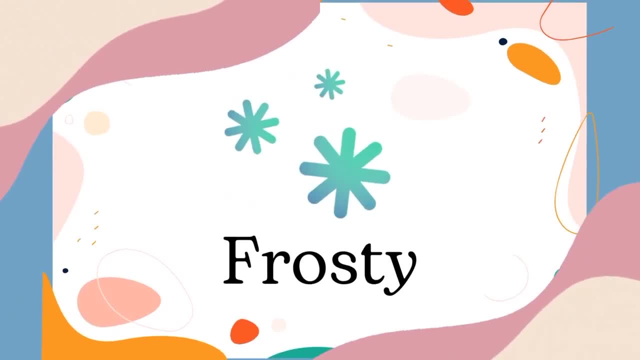 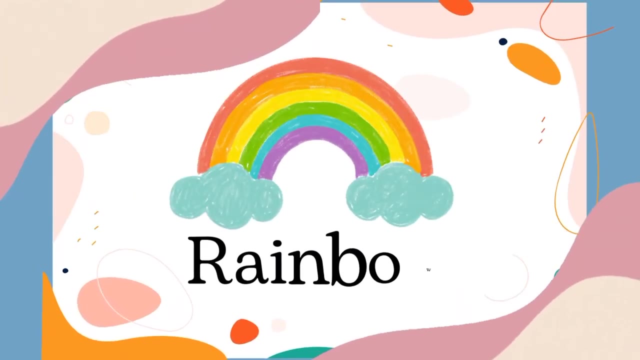 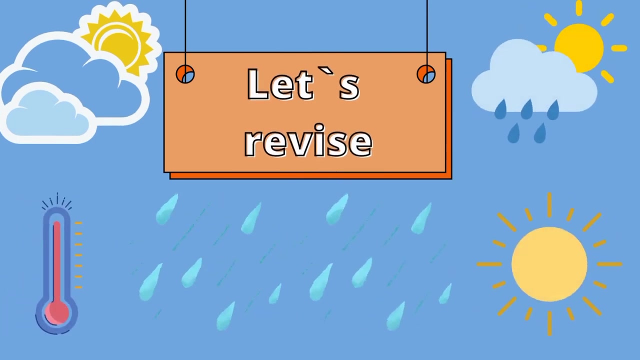 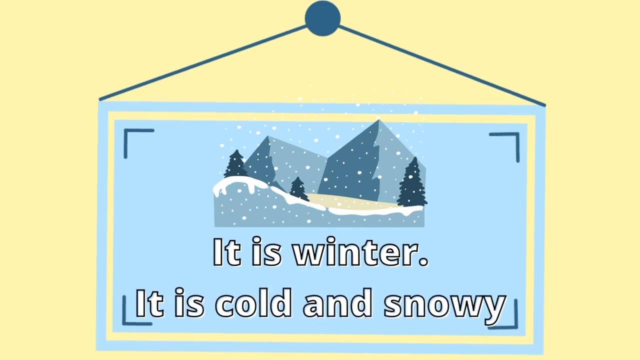 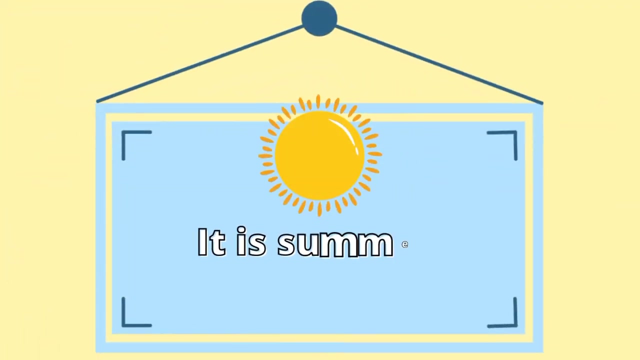 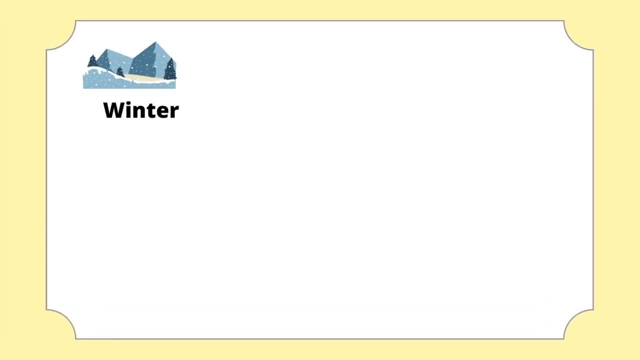 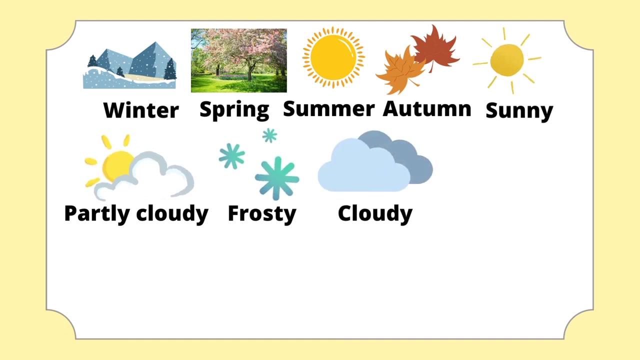 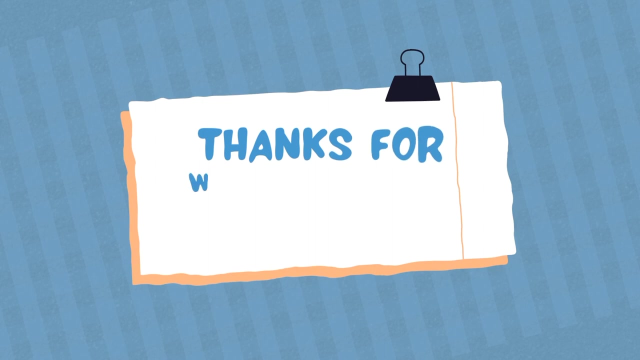 cloudy, winter, spring, summer, autumn, sunny, hotly cloudy, frosty, cloudy, foggy, cold, hot, snowy, rainy, rainbow. thanks for watching my video. please subscribe to my channel and click on the bell to get notifications for new videos every week. subscribe.